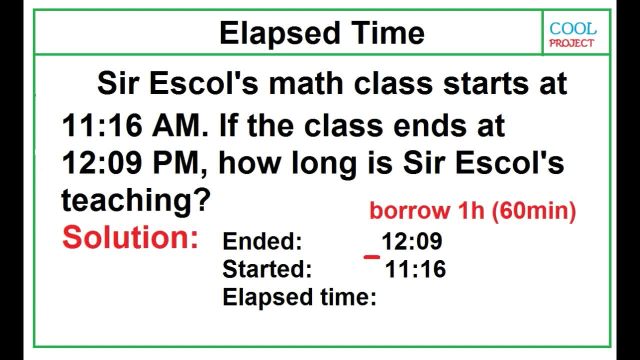 Knowing that 1 hour is equal to 60 minutes, let's add 60 minutes to 9.. 12.09 becomes 11.69.. Now we can subtract 11.16.. The difference is 53.. The answer is 53 minutes. 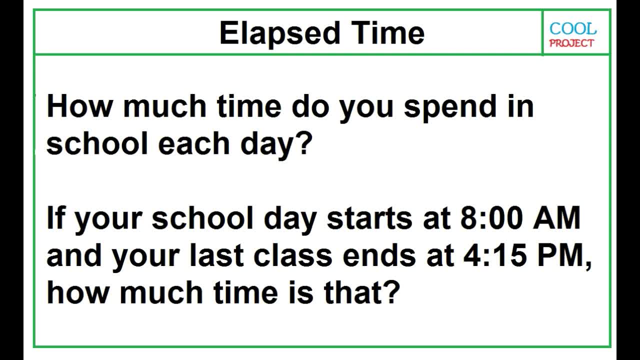 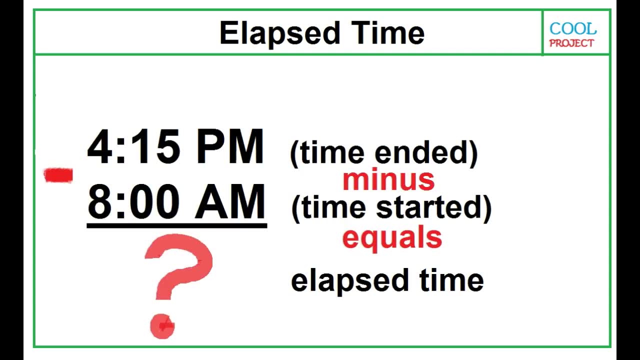 Another example: How much time do you spend at school each day? If your school day starts at 8 am and your last class ends at 4.15 pm, how much time is that? Again, just find the difference. 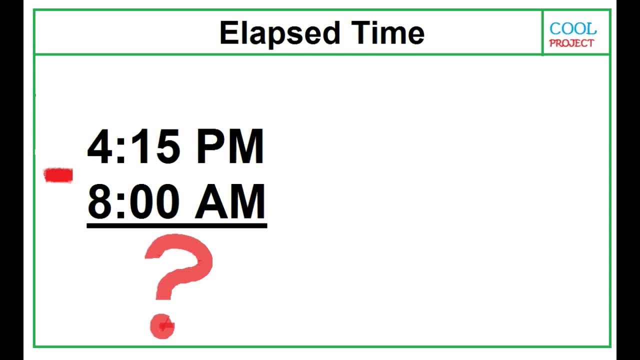 4.15 minus 8 is The elapsed time. Since we cannot immediately subtract 8 am from 4.15 pm, rewrite 4.15 pm to its equivalent number of hours by adding 12.. 4.15 pm is just equal to 16 hours and 15 minutes. 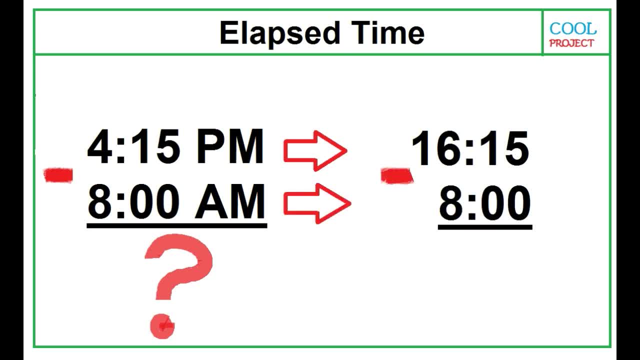 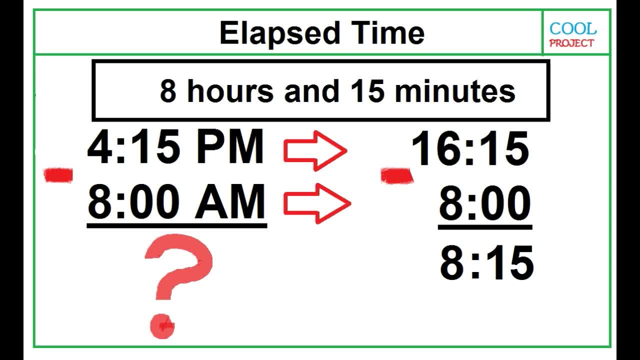 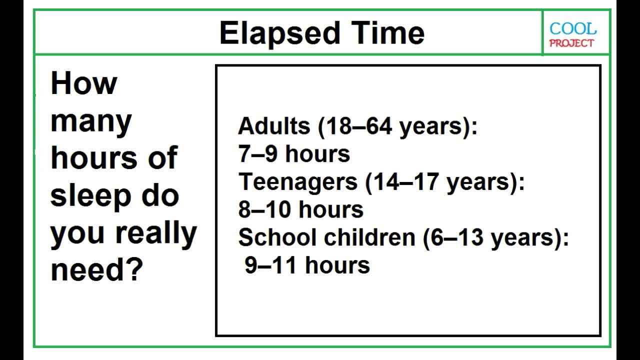 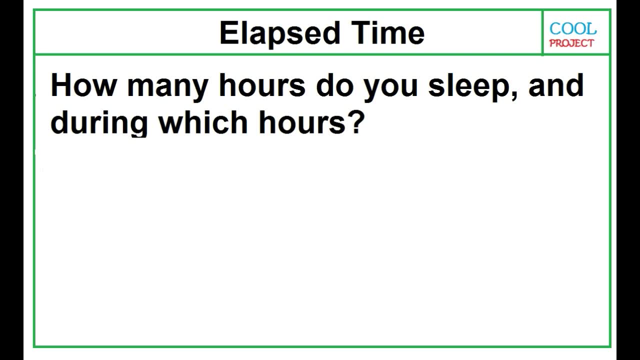 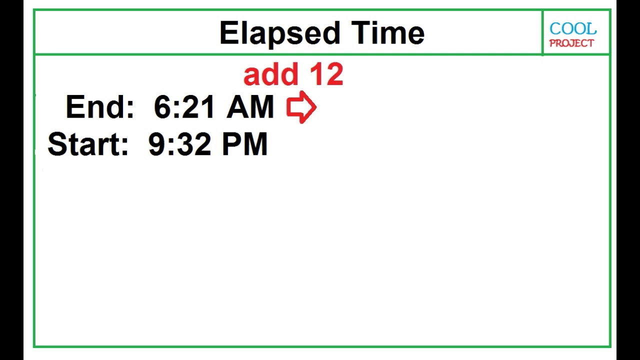 8 hours and 15 minutes. How many hours of sleep do you really need? How many hours do you sleep, and during which hours? Ok, let's find the difference: 6.21 am minus 9.32 pm From 12 noon. 6.21 am is 18 hours and 21 minutes.